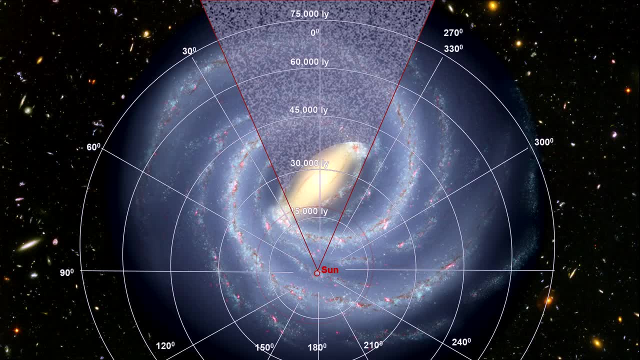 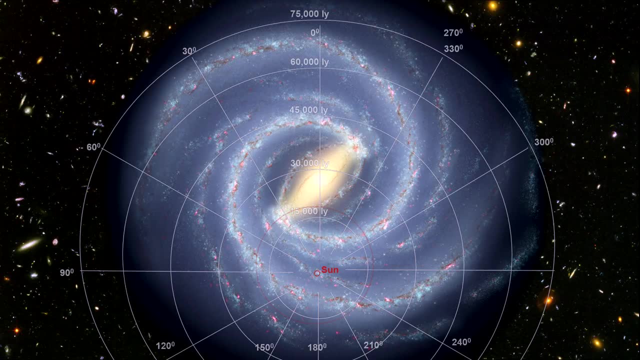 But our understanding of spiral galaxies is that they are symmetric, So this picture makes that assumption and fills in the blanks accordingly. Here we see the Sun's orbit around the galactic center. Our orbital speed is approximately 230 kilometers per second, or 143 miles per second. 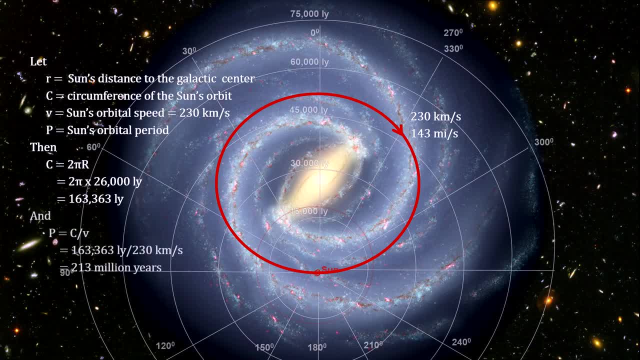 That's fast, but it takes us around 213 million years to complete one orbit around the galactic center. The last time we were in the same place in our orbit, dinosaurs were just starting to appear on the Earth And we have traveled around one ten-thousandth of a revolution since the origin of humans. 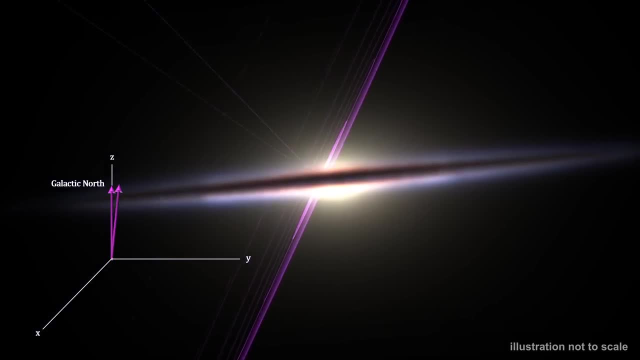 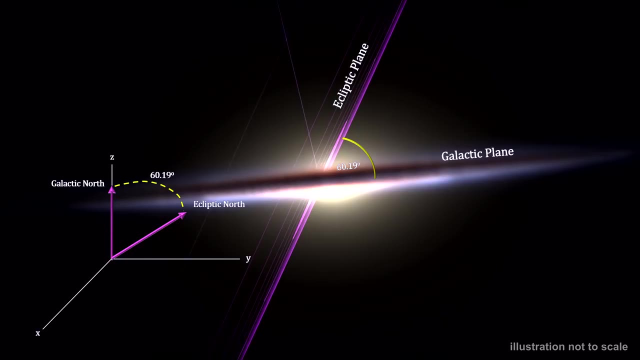 Here's a look at our Solar System. This is the solar system's ecliptic plane. with respect to the galactic plane, It's just over 60 degrees off. We see that the solar system is quite out of alignment with the galaxy's disk. 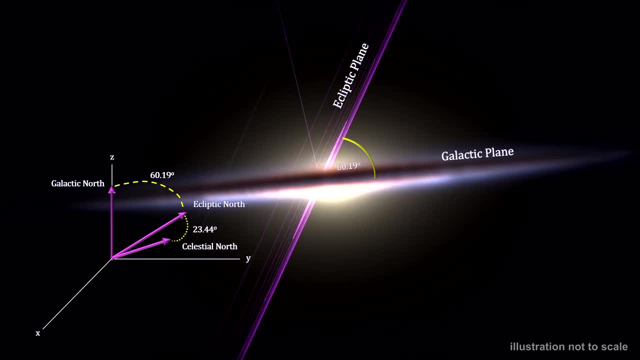 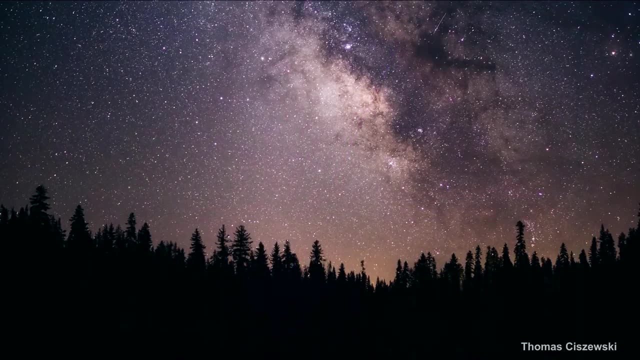 Earth's 23-degree tilt to the solar plane puts us at an almost 63-degree tilt from the galactic plane. This is why the Milky Way appears at such a strange angle. This is why the Milky Way appears at such a strange angle. 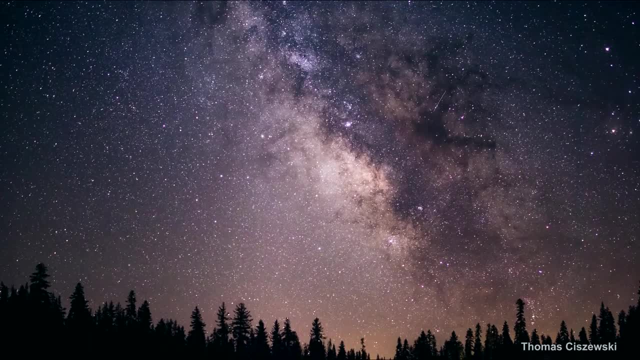 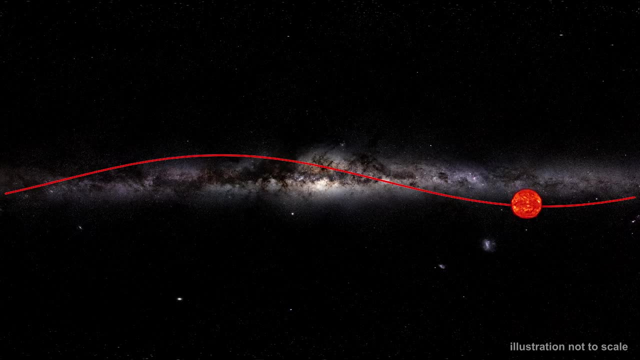 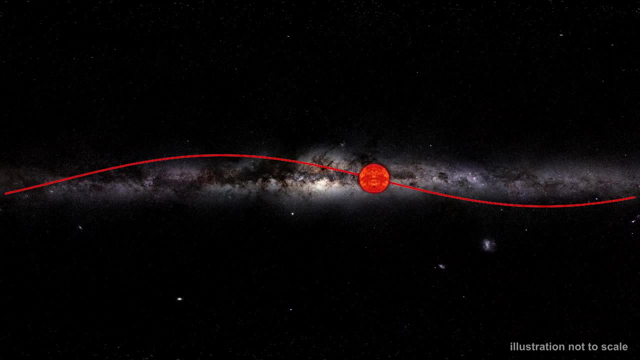 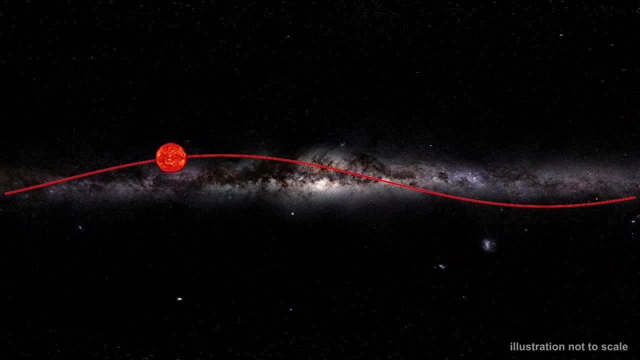 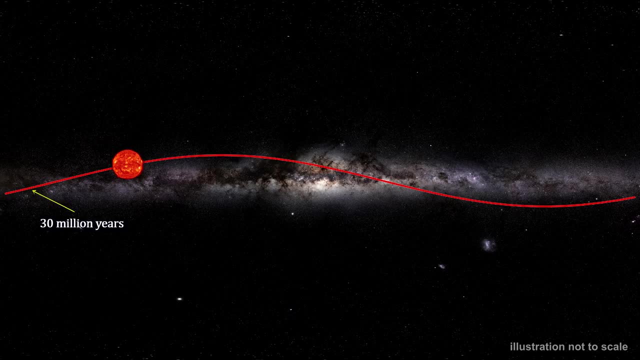 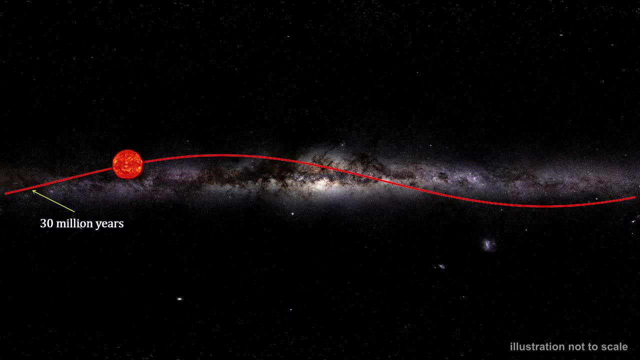